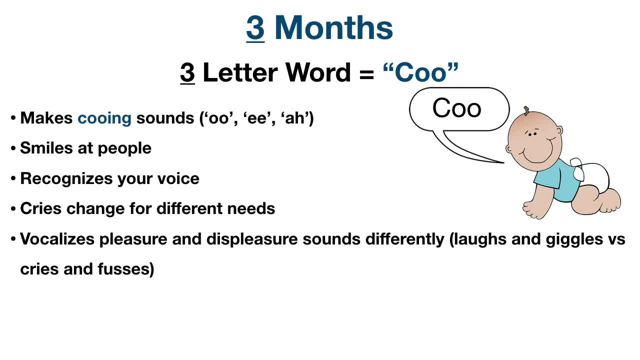 For example, they laugh and giggle as a way to communicate happiness and they cry and fuss as a way to communicate when they're upset. I do want to point out that, as we walk through these different milestones, remember that they're average time frames and that some milestones can occur. 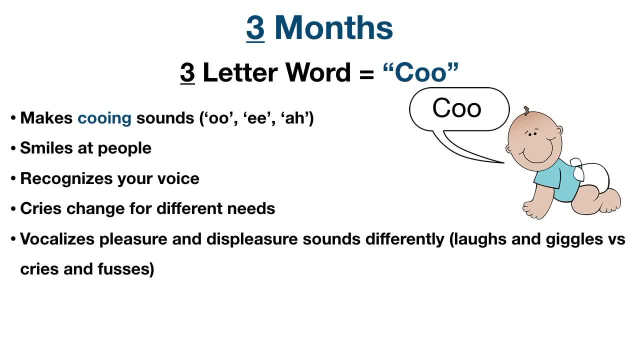 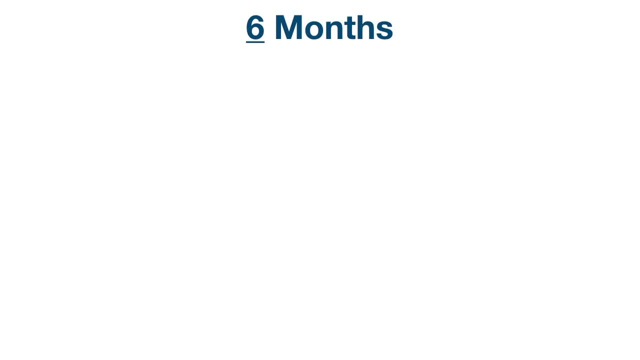 sooner or later, But for the purposes of this video, these are the milestone time frames that may come up on medical exams. Next we have six months. Again, we're going to use the age to remember the milestone. So for six months, remember the six-letter word babble. By this age, the infant. 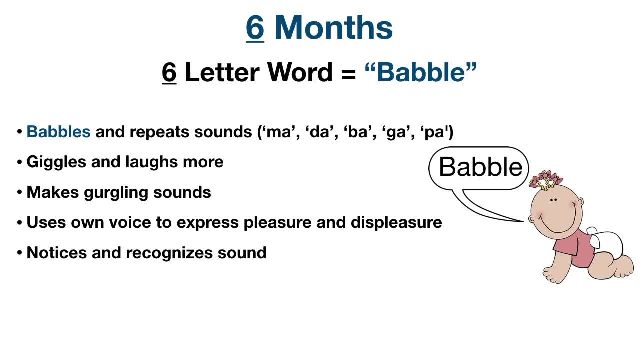 starts to babble and repeat sounds. They may babble mama or dada without much meaning, and that's because the repetitive consonant sounds they tend to produce first when babbling are b, d, g, m, p and t. The infant will also continue to giggle and laugh more. They'll start to make gurgling noises. 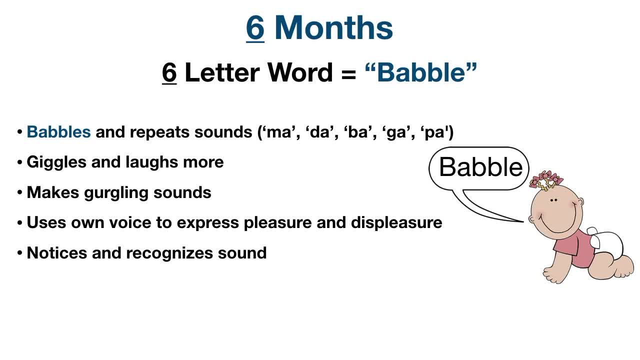 and they will also use their own voice to express pleasure and displeasure. This is different from three months. Remember, at three months they would use laughing, crying and fussing to vocalize and communicate pleasure versus displeasure. Well, by six months they may start to use their own voice and use speech like babbling sounds to. 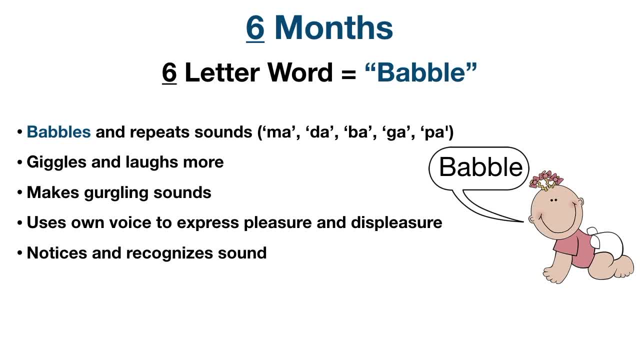 express when they're happy or upset. Finally, the infant notices and recognizes sounds more. They may move their eyes in the direction towards sound, They may pay attention to music and they respond to changes in the tone of your voice. Moving on to nine months, we're going to use the 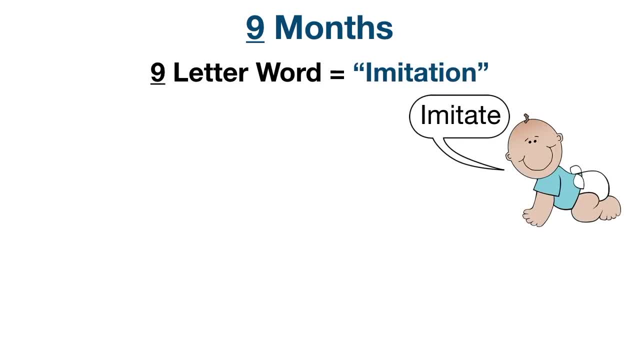 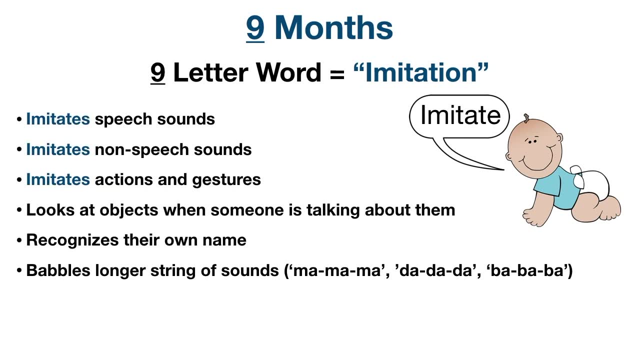 age again to remember the milestone. The nine-letter word to remember for nine months is imitation. This is the start of the baby's imitation phase. Imitate speech and non-speech sounds. They will also imitate actions and gestures. They may gesture. 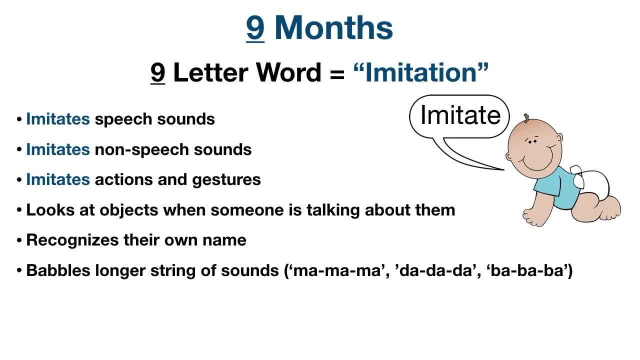 without being prompted to. by pointing to objects and showing them to others, They also look at familiar objects. when someone is talking about them and the infant starts to recognize their own name, The baby's babbling increases and they start to string longer babbling sounds together. 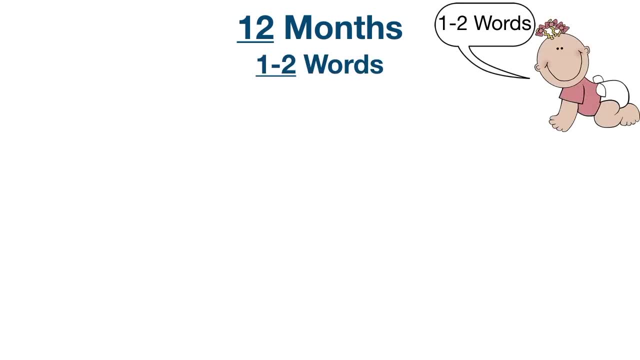 Next is 12 months of age and using the age, we're going to take- the 1 and 2 and 12- to remember one to two words. By 12 months of age the child usually can say one to two words. This could be in addition to mama and dada, and their vocabulary could be even. 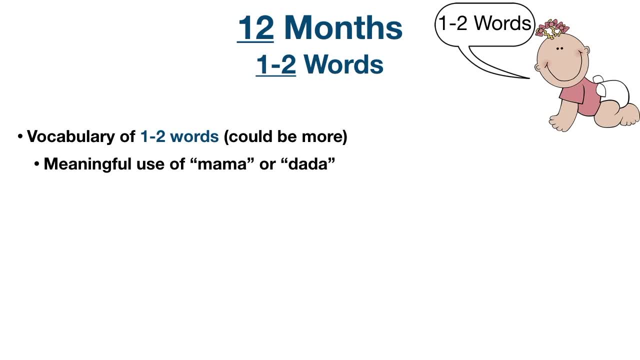 larger, depending on the child. Their use of mama and dada has more meaning to it now. Remember, during the babble phase they can say mama and dada without much meaning. However, by 12 months of age they start to bring meaning to it. You can also think of the 12-month milestone as the understanding phase. 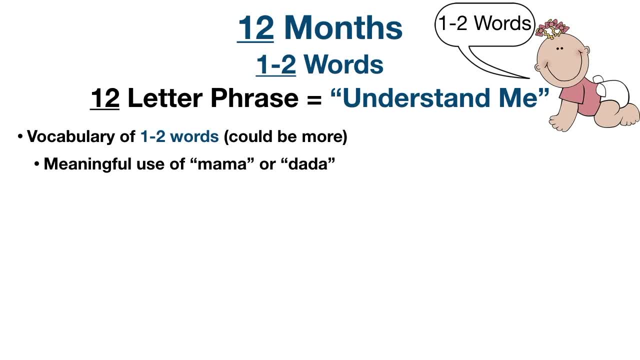 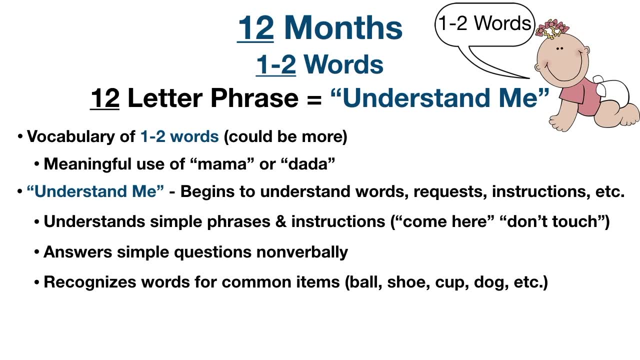 and you can remember that using the 12-letter phrase. understand me. They begin to understand anywhere from three to fifty words. They begin to bring meaning to their vocabulary And they begin to understand simple phrases, instructions, requests and commands such as put. 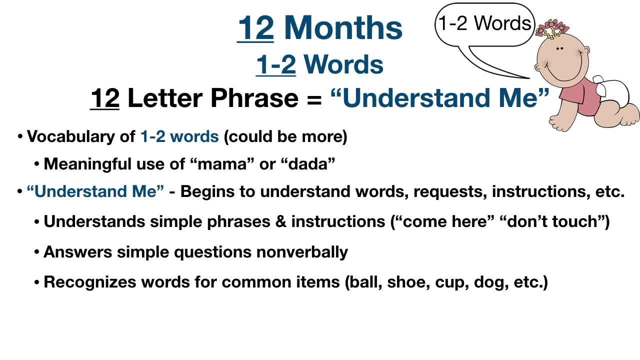 the toy on the ground. come here and don't touch Along those same lines. the child may start to understand and answer simple questions non-verbally by nodding and shaking their head, Or they might go to get an object when requested to do so, which makes sense because again, they're starting to. 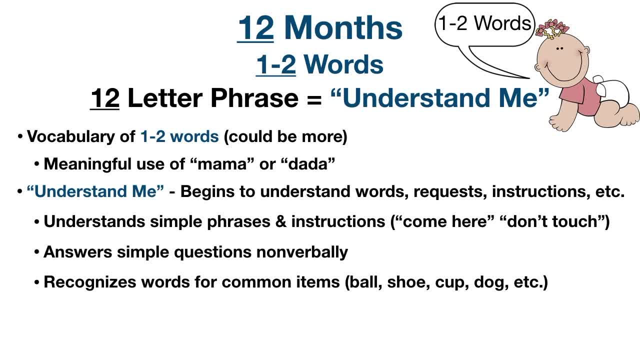 understand simple instructions, as mentioned before. Finally, they understand and recognize the names and words for common items such as ball, shoe, cup, juice and dog. This understanding phase is a process and everything listed here won't happen right at 12 months of age. However, 12 months is when they start to develop these speech and 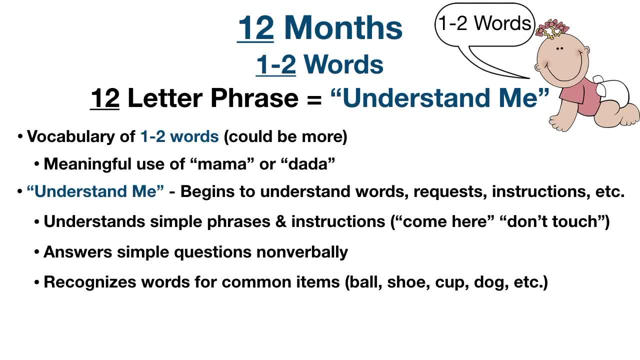 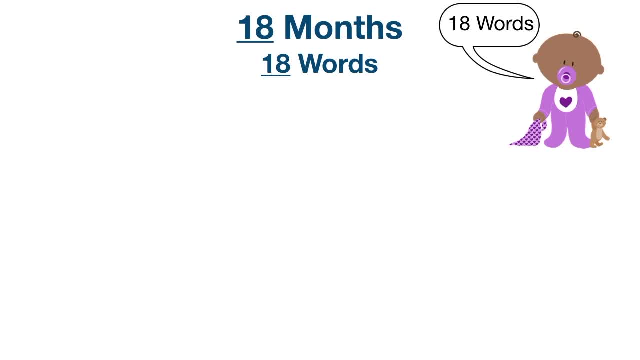 language skills and they continue to develop those skills throughout their second year of life. As we move on to 18 months, we can again use the age to remember the milestone of 18 words. This will help you remember that by 18 months the child, on average, will have a vocabulary of 10 to 20. 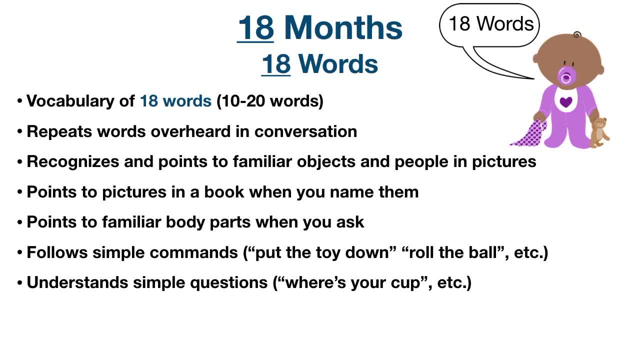 words. Around 18 months or soon after, the child may have a vocabulary of 10 to 20 words. The child may have a word spurt in which their vocabulary drastically increases to 50 words. The child also starts to repeat words overheard in conversation. They also become more interactive with their 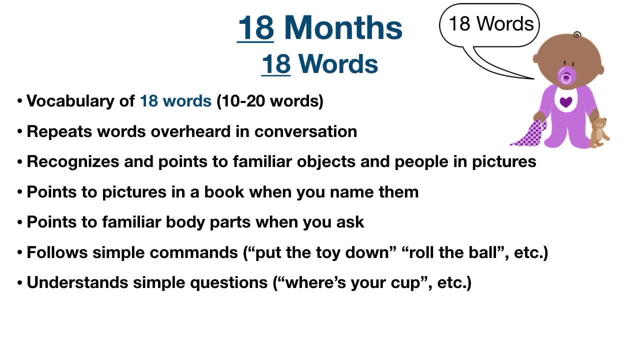 understanding. They recognize and point to familiar objects and people in pictures. They point to pictures in a book when you name them and they point to familiar body parts like eyes, ears and nose when you ask. As we mentioned before, with 12 months they continue to develop. 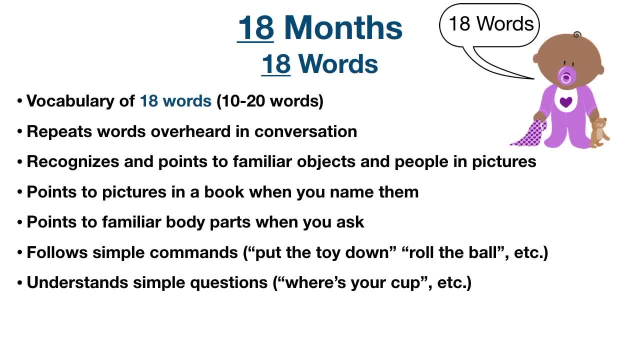 their understanding and ability to follow simple commands like put the toy down or roll the ball, And they continue to understand more simple questions like where's your cup or where are your shoes? Next, we have two years of age. The two can be used to remember the milestone of two word phrases. 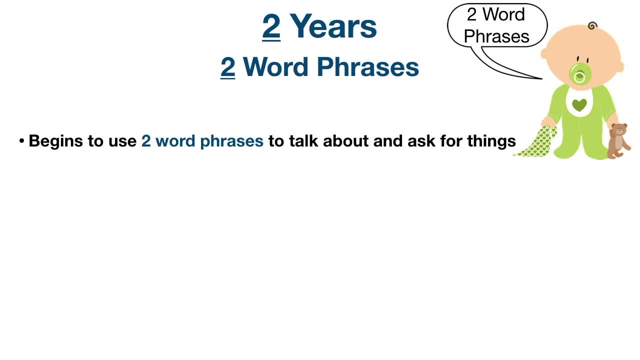 The child would begin to use two word phrases in order to talk about or ask for things. They will put two words together, like more milk, no juice or daddy book, And they will ask two word questions like where's doggy, where's kitty, go bye-bye or what's that? Keeping in line with 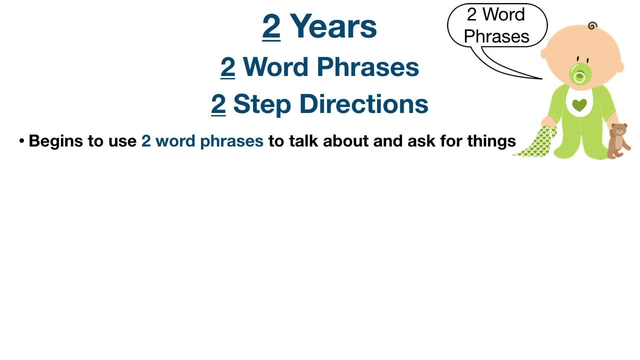 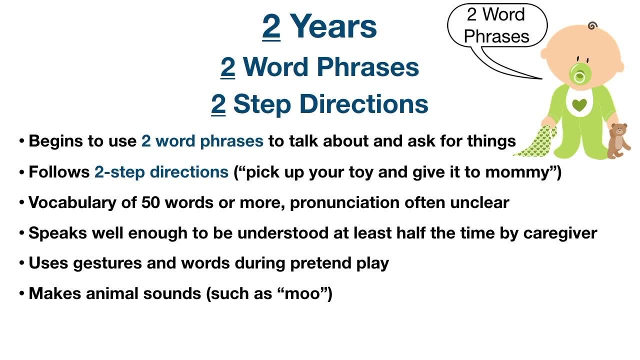 using the number two. you can remember that by two years of age they will be able to remember the two word phrases. We'll start following two step directions, such as pick up your toy and give it to mommy. They may have a vocabulary of 50 words or more. however, the pronunciation is often unclear. 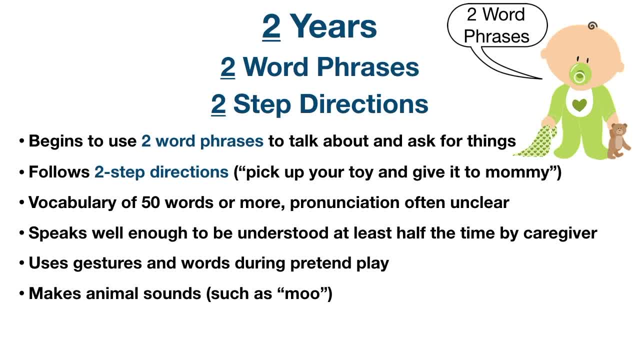 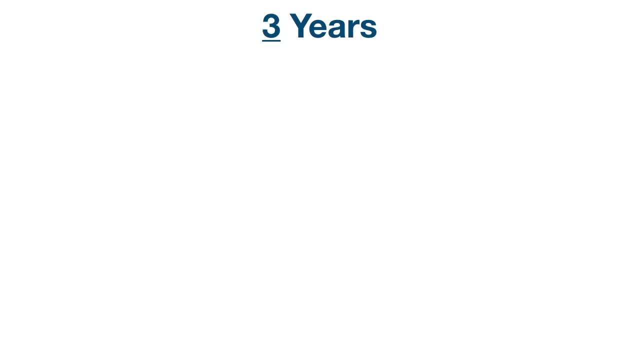 The parents and primary caregiver usually can understand at least half of the speech. The child may also use gestures and words during pretend play and they also start to make animal sounds. Moving on to three years old, we can use a similar trick as we did for two to remember two. 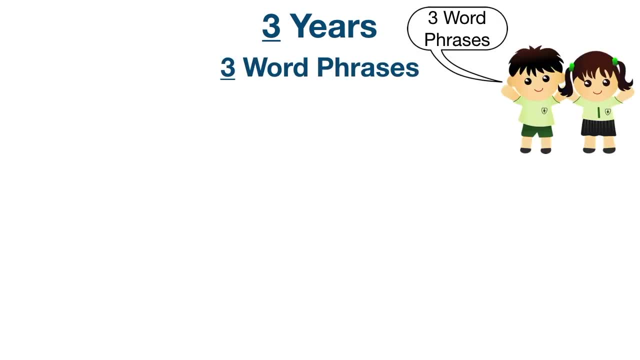 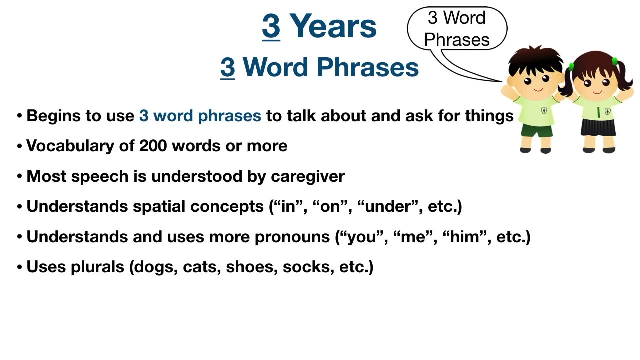 word phrases. Now, for three years old, we'll remember three word phrases. The child will begin to use three word phrases in order to talk about and ask for things. By age three, the vocabulary can be 200 words or more. and not only does their vocabulary expand. 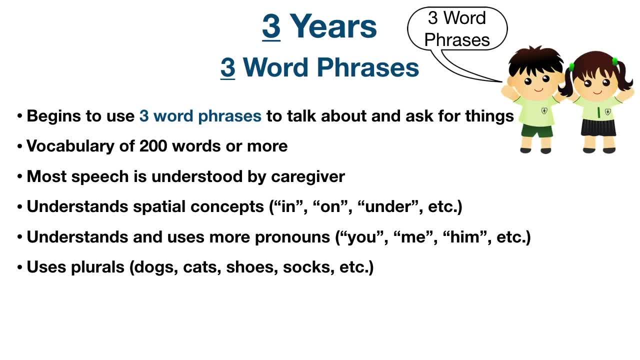 but their grammar and pronunciation also improve. Their speech becomes more clear, especially to the parents or primary caregiver. They begin to ask what and where type questions, and they understand spatial concepts such as in, on or under, as well as concepts involving different colors and time. 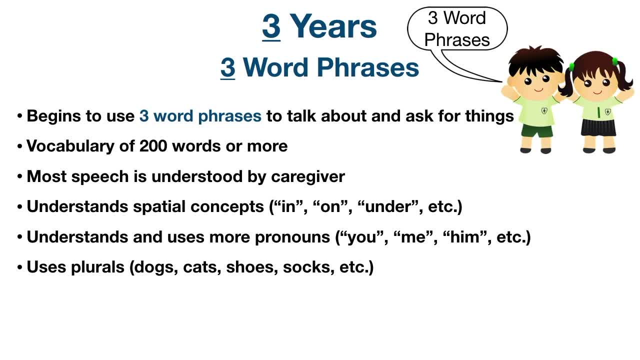 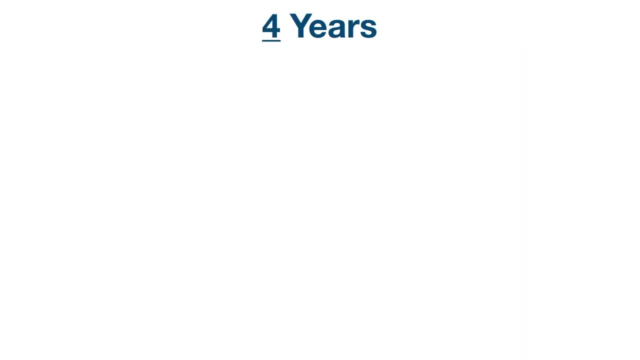 The child will understand and use more pronouns such as you, he, him or her, and they will also understand and use plurals such as cats, dogs, shoes and socks. Finally, we have four years old. The trick to remember this milestone is four or more word. 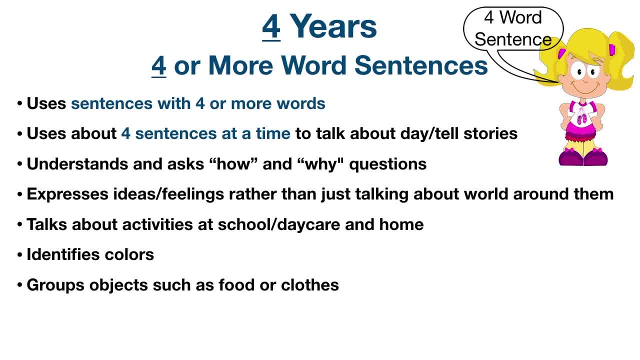 sentences. The child will use sentences with at least four words and they will also use four or more sentences at a time when talking about their day or telling a story. They have a deeper understanding of more abstract concepts and will understand and ask how and why- type questions. 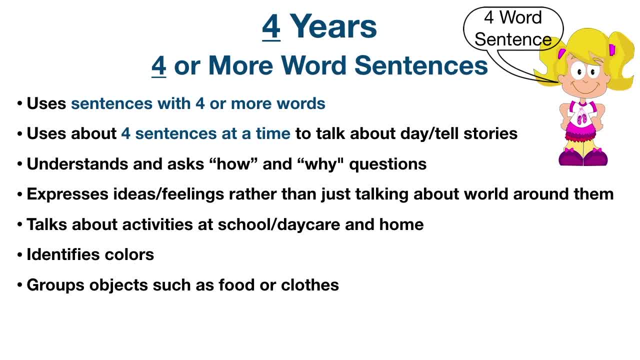 Along those same lines, they will start to express their ideas and feelings. rather than just talking about the world around them, They talk more about their day and activities at school, daycare or home. Parents and caregivers will understand most, if not all, of their speech. 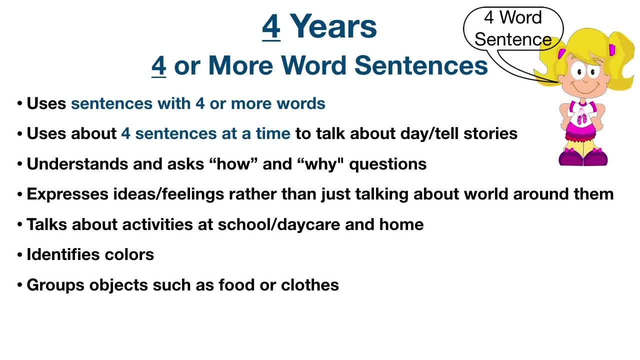 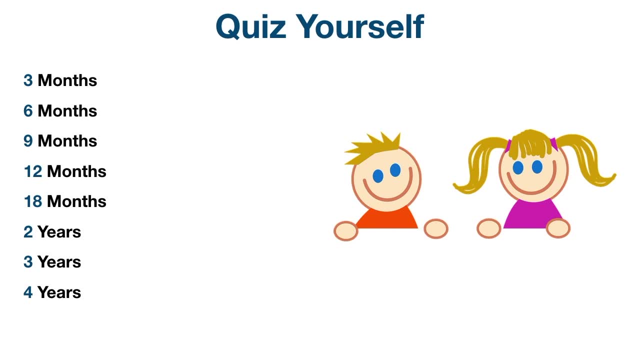 and strangers can typically understand the child without much difficulty. They typically can identify colors by this age- and this often happens even sooner- and they can usually group objects into different categories, such as food or clothes. Now it's time to quiz yourself and see if you can name the milestone trick that correlates with each age. 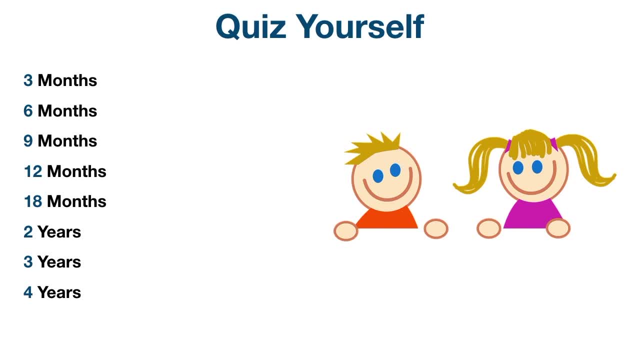 Starting with three months. what did we say was the trick to remember? It was the three letter word coo, to help you remember the infant coos at this age. So for three months, always think of the word coo. Moving on to six months of age, what did we say? 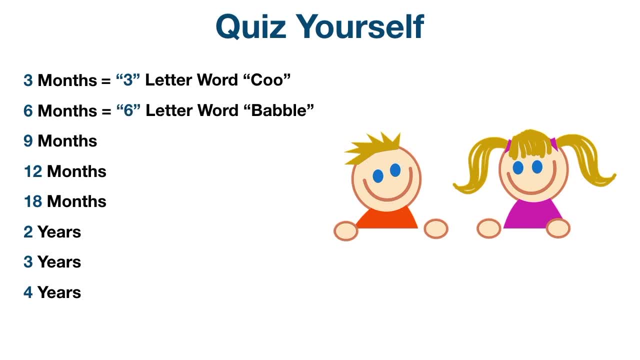 the trick was. It was the six letter word, babble, to help you remember the infant babbles at this age. So for six months, always think of the word babble. Next is nine months. Try to name the trick for this. You're going to use the nine letter word, imitation, and this will help you remember the imitation phase. 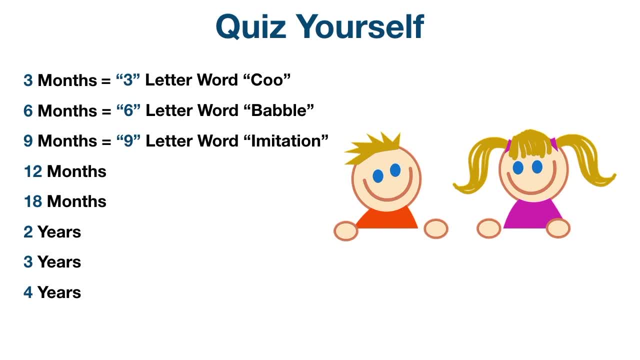 in which they imitate speech and non-speech, sounds, actions and gestures. So, for nine months, always think of imitation. Moving on to 12 months. what did we say? the trick was: You're going to take the one and two in 12 months to help you remember one to two words. 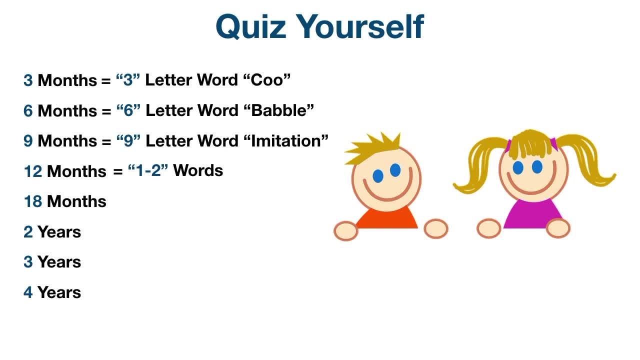 The child has a vocabulary of one to two words, usually in addition to mama and dada. You can also use the 12 to remember the 12 letter phrase. understand me and this will help you remember. the child starts to understand words, requests, instructions, commands and questions. 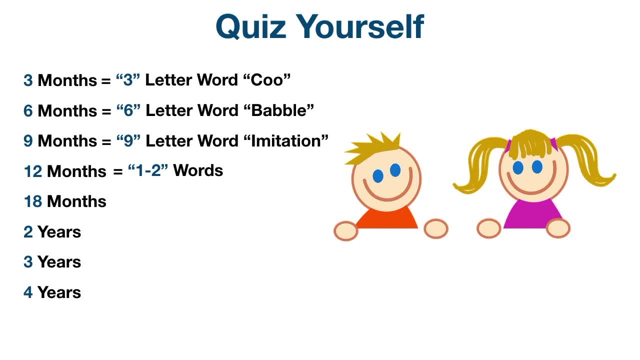 As we progress to 18 months. name the trick for this? It's 18 words, which will help you remember that they have a vocabulary of 10 to 20 words, which rapidly increases to 50 or more words as they approach two years old. Next we have two years of age, so what's the trick for this? 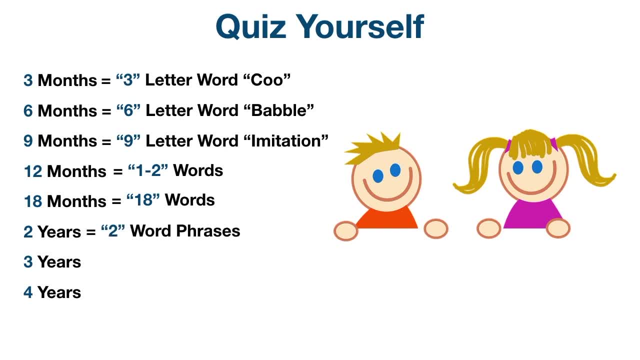 The trick to remember is two word phrases, which will help you recall that by two years of age, the child starts to put two words together in order to talk about or ask for things. The two can also be used to remember two-step directions, and this will help. 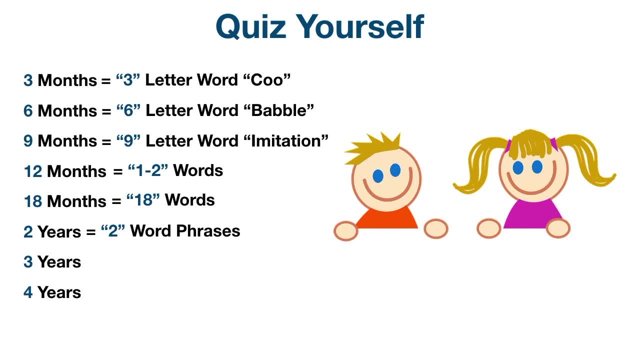 you remember the two-step directions and this will help you remember the two-step directions. you recall that the child can understand and respond to two-step instructions. Moving on to three years old. what's the milestone? The trick to remember is three word phrases.